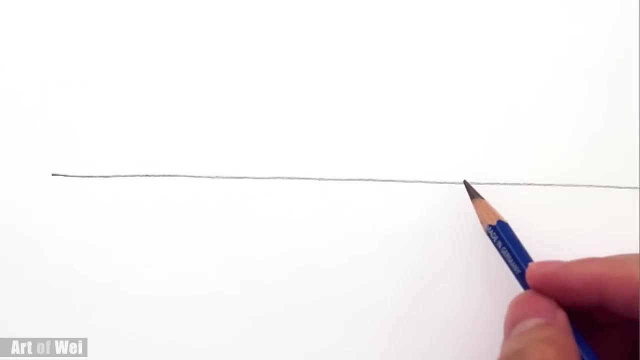 it's kind of like looking now into the ocean. right, you see the horizon line. So with this horizon line, um, this is I'm going to start out with a one point perspective. so this is kind of like the the most simple, uh simple- perspective that you can get. so it's just one point. 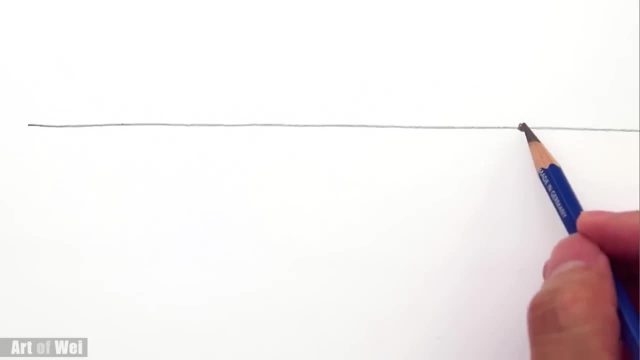 So, basically, one point means that you're going to have one point on the horizon line and then if you create these lines like this, you know now you're getting perspective. uh, coming from this one point here. So with these lines, let's say, you want to just draw like a box. 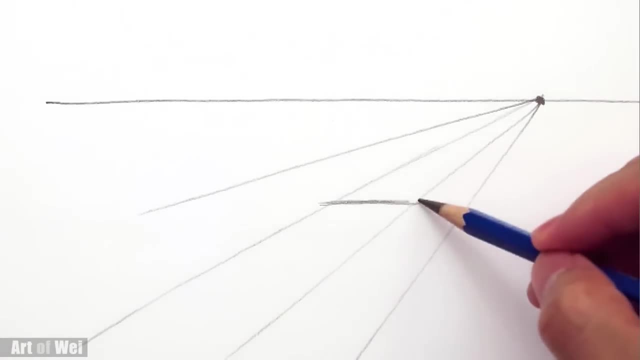 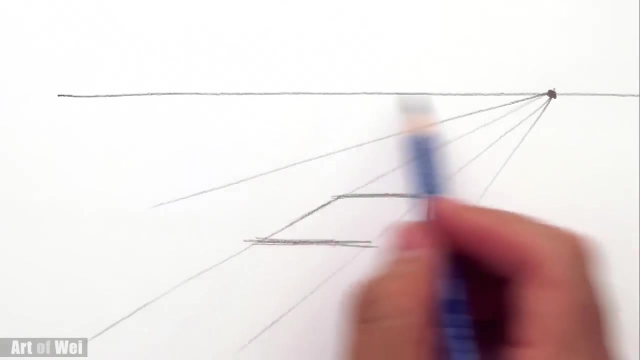 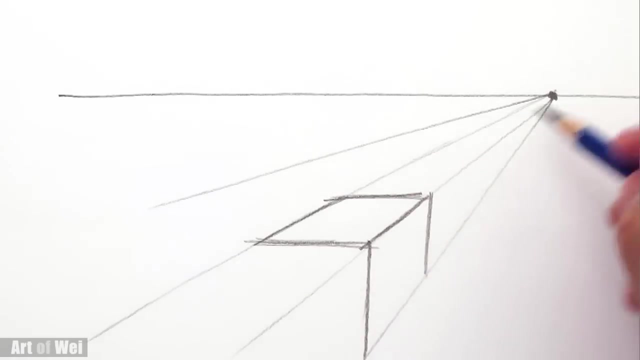 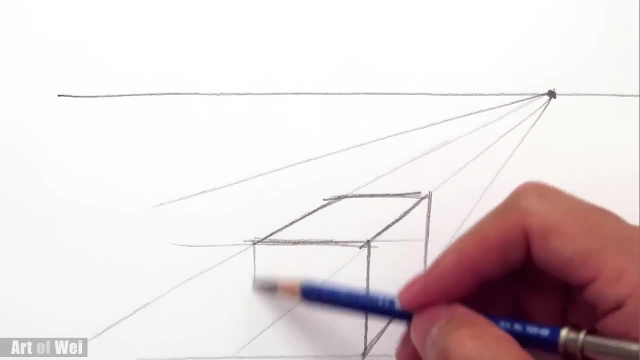 so with these perspective lines, you can actually do. let's just say something like this: okay, and these all these lines right here will be parallel to the horizon, so there's only really, um, the other perspective line is going in one direction. okay, so we can do so. all these lines are parallel and this is kind of like perpendicular, right. so 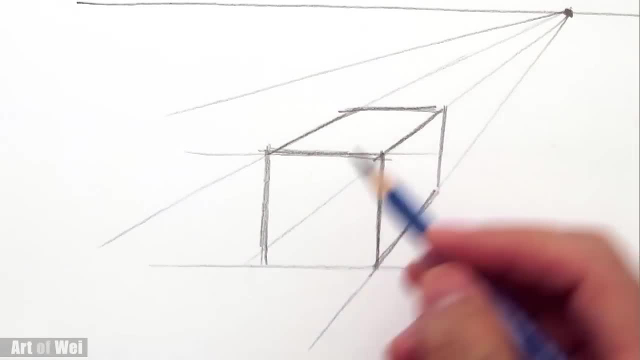 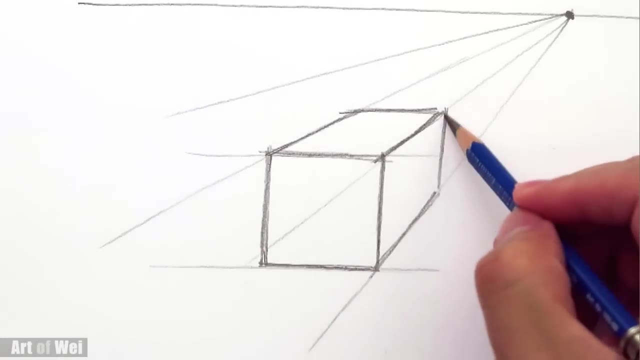 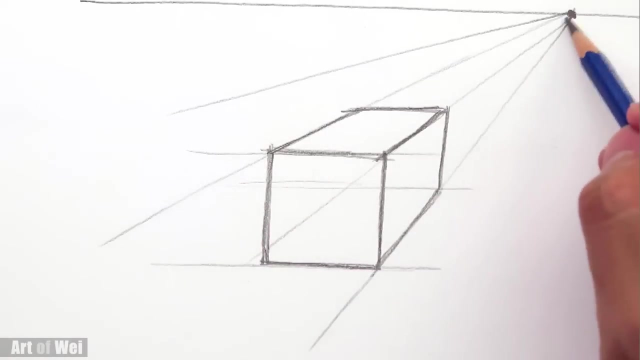 it's perpendicular to the horizon. so this is what they call one point perspective, and if you want to visualize this box, you know, let's say a little bit better, uh, very useful. I'm going to draw the back of this. so these lines will be connecting all the way, all the way to that point. 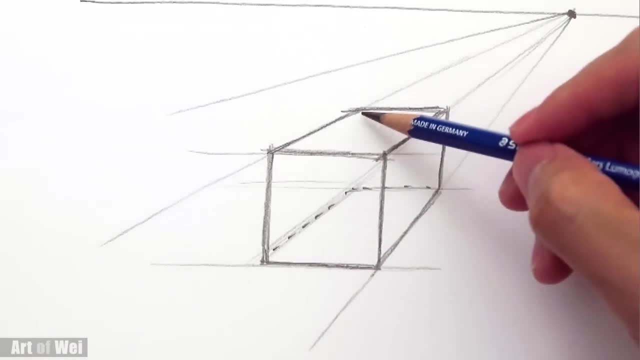 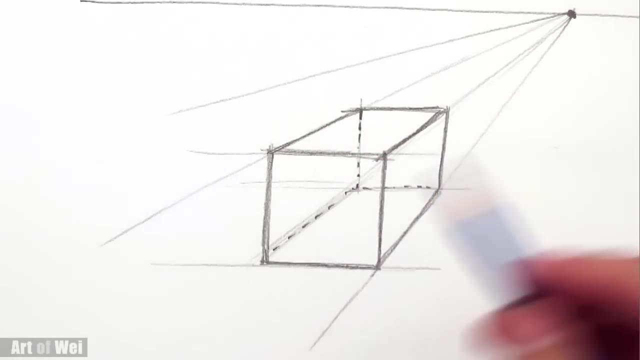 so this would be the back of the box. and why am I drawing this back of the box? because it's- uh, you know, in drawing in general, it's always good to be able to visualize things behind. so that's why, um, I'm just kind of drawing this just for the just for the heck of it, okay, so this? 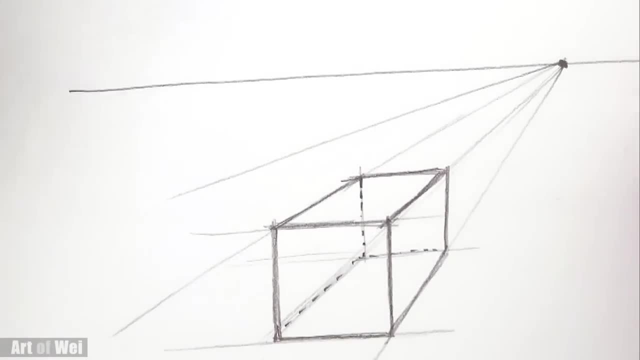 would be a one point perspective. so this is the most basic form, and let's move on to two point perspective. so let's see, let's draw the horizon line again. okay, so with two point perspective, that's what it is. it's just two points. so instead of one, I'm gonna have two. okay, so let's just 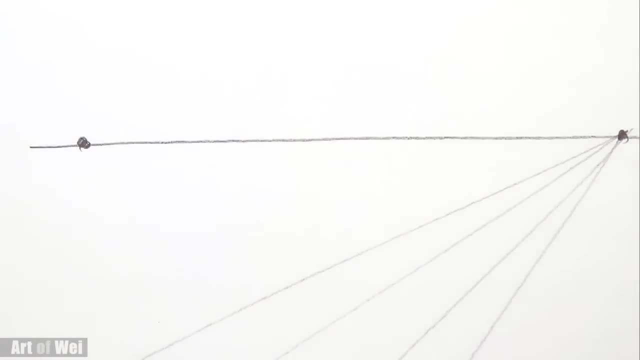 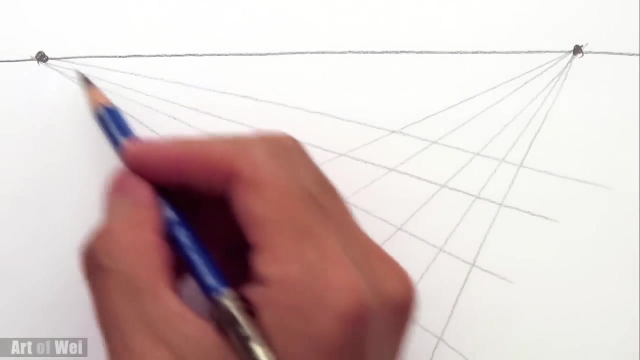 connect these lines a little bit, just draw some guidelines. yeah, okay, I'm gonna do another one here, and what this gives you it's, you know, it's kind of like a three-dimensional grid. now. right, like, instead of just parallel lines, now we actually have um, two perspective lines. so let's say you want to do a box and I'm just 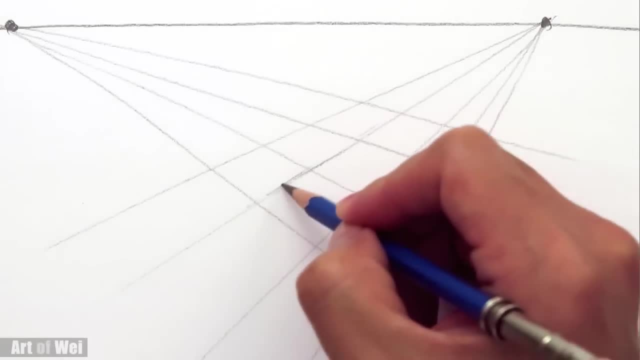 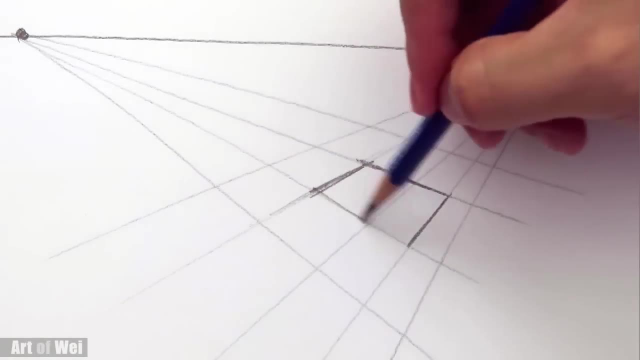 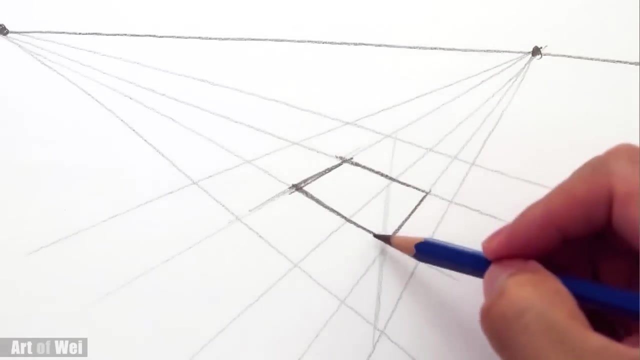 gonna take one of these lines, for example. so let's draw. let's draw like a smaller one, since we're here. so let's say, this would be the, let's say, the top of the box. that's a little bit smaller now. these lines are still vertical, okay, so these are still perpendicular to the horizon. 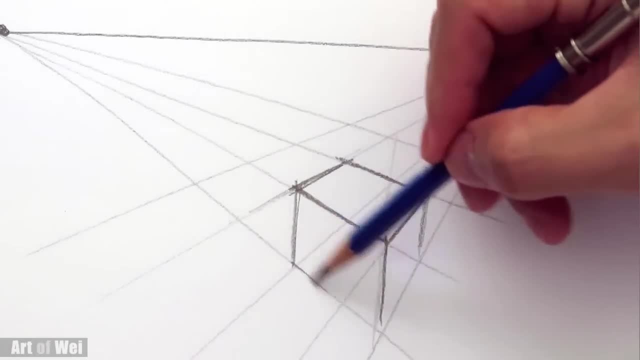 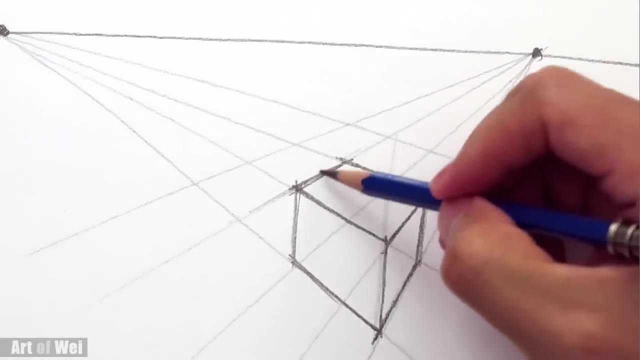 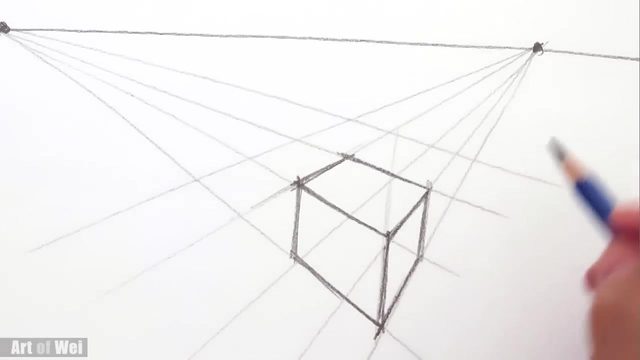 so I'm just kind of let's, let's make this as the base of the box and then let's connect this. okay, so with two points perspective, now what you're getting is some it's a little bit more realism. there's a little bit of warping right, because you know, this is kind of a very wide 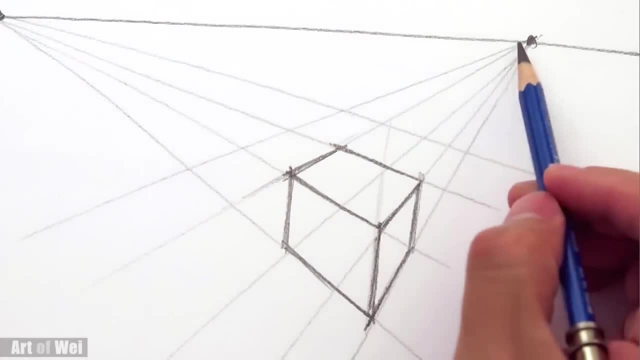 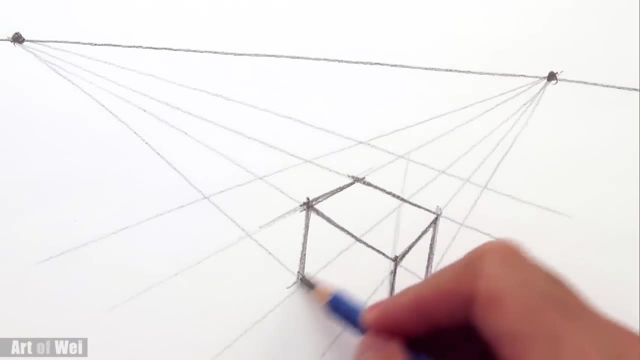 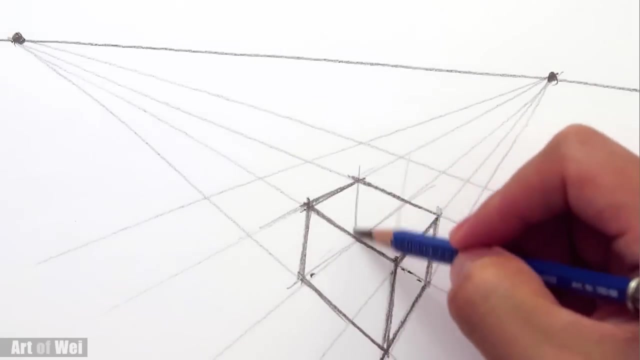 angle, because the uh, the uh, the vanishing points here are fairly close together, so you're gonna get a very wide angle. so this, this thing almost looks like it's being distorted. okay, so let's say we're going to draw the back of this. well, actually the back is going to be. this is still vertical. 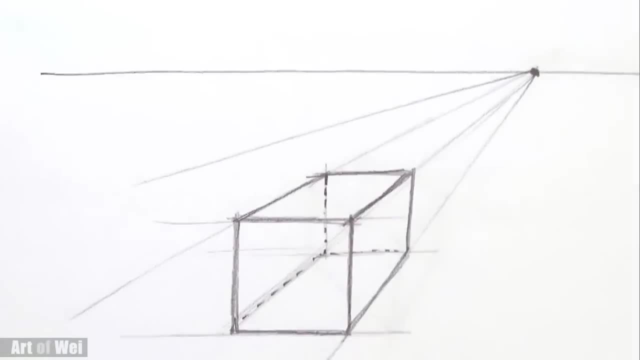 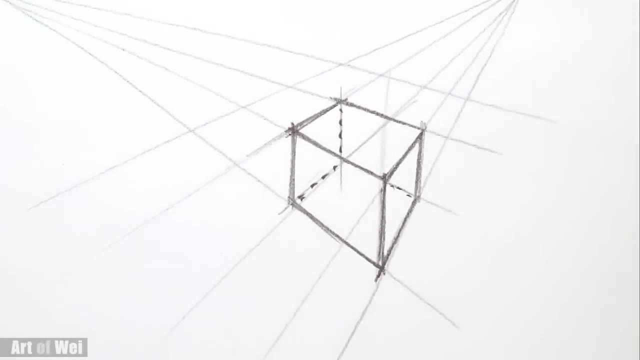 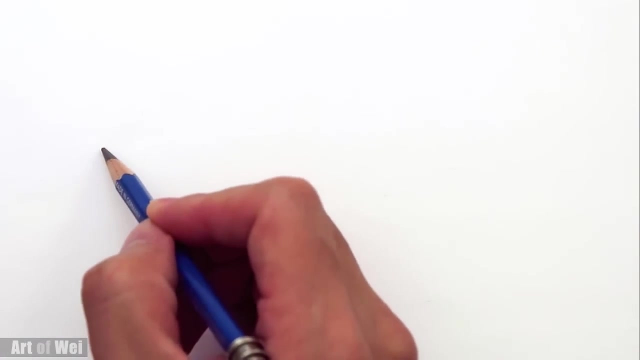 okay, so this would be your two points perspective, compared to this being the one point perspective. so we see how simple this is compared to this, right, but this one feels a lot more. you know, just three-dimensional in general. all right, so let's add more, and this is what they call a three-point perspective, and it's actually not that useful. 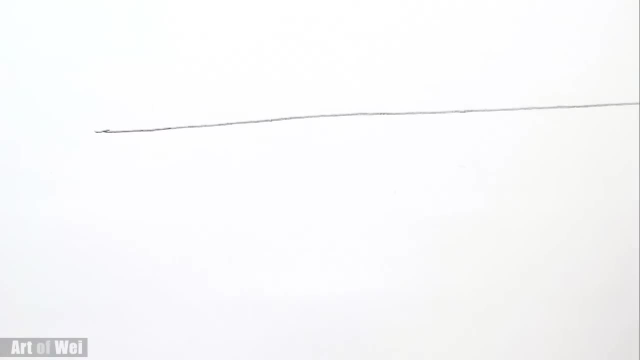 for general purpose drawing, because it's a little bit too complicated. so just let me go over real quick. so here's two points right, two vanishing points right here. so we have these grid lines. let's just make a couple of lines where you can see- and i'm just kind of going over this- 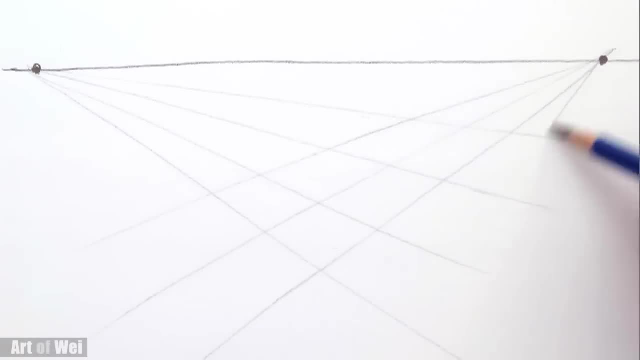 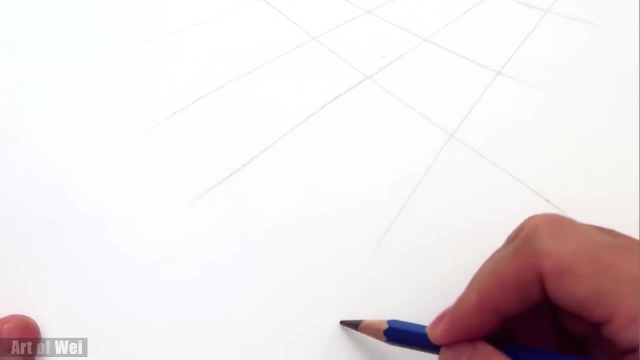 just so I can show you- so you have a little bit of knowledge on three point perspective- that I don't really use this that much at all. um, all right, so with three point perspective point, there's got to be another point, and I'm going to put it right at the bottom here. okay, 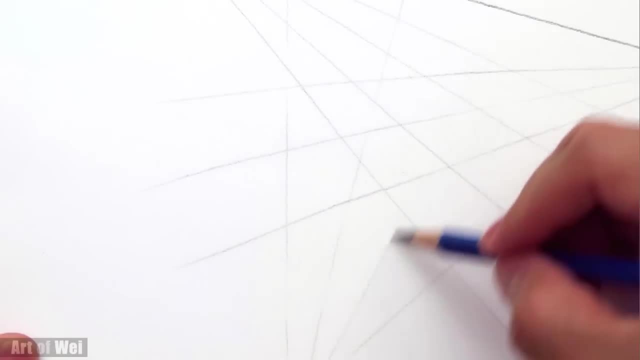 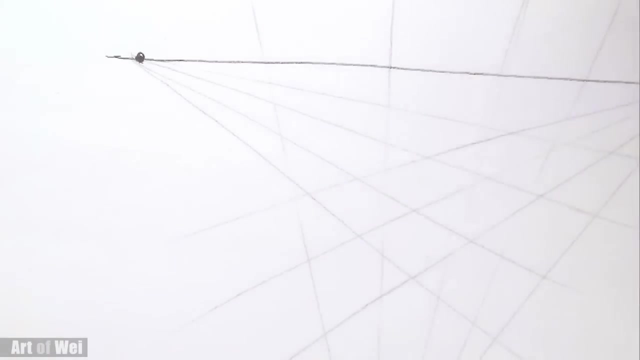 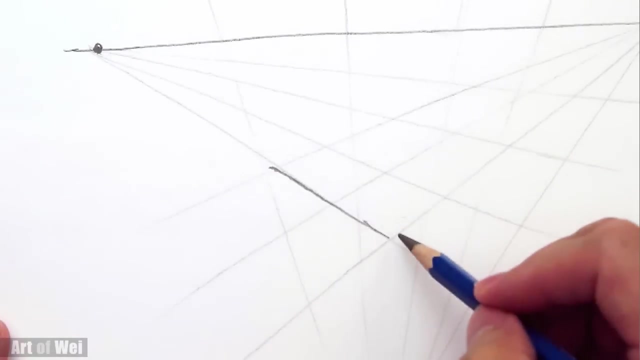 so I'm going to make some lines here and this kind of stuff. perspective would be good if you're doing like you know, like a bird's eye view, you know, maybe it's standing on top of a building or something. so let's just say I want to do a little box and this would be the base. okay, so let's just 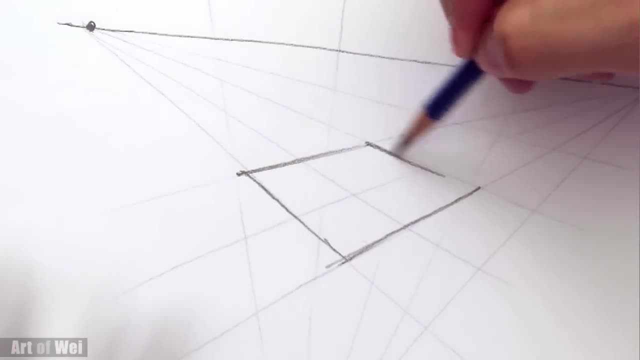 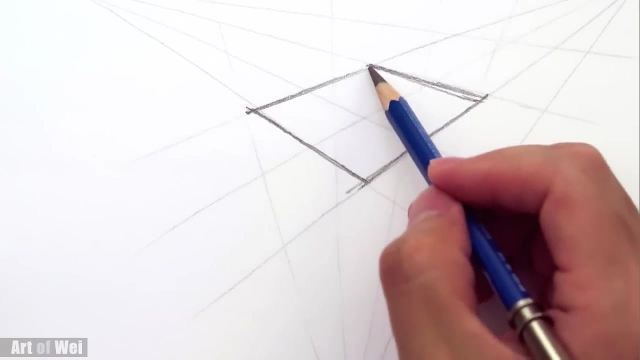 do this, I'm just going to use this: this is the going to be the bottom. actually, this could be the top. let's do the top then. all right, so with three point perspective. you know, here let's say: this is a rooftop, right? so this is two points. and then with three point, we're going to add in this: 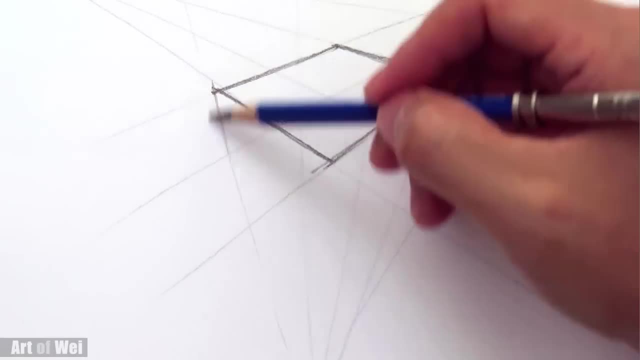 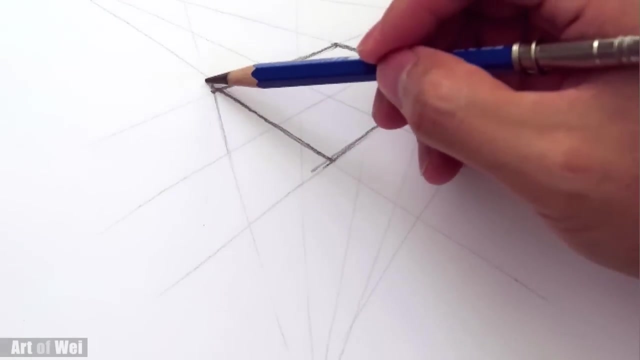 point here. so now we're going to follow these lines. so, instead of having a vertical, you know, whereas we have in the two point perspective and one point, everything was was vertical, this one's actually going to move down to the point here too, you. so these are going to give you these lines right here. 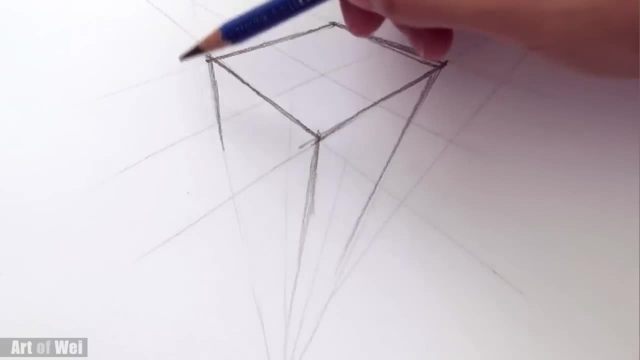 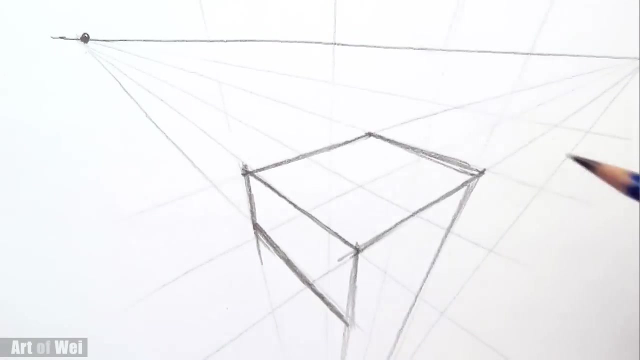 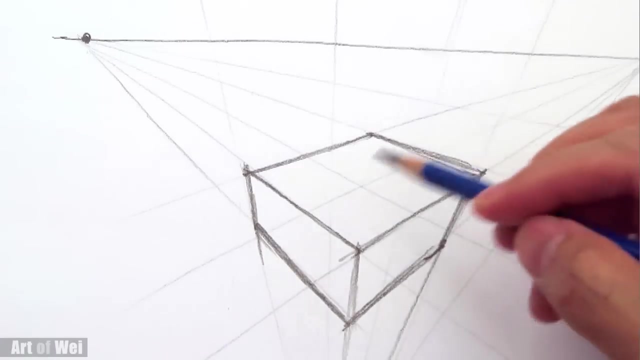 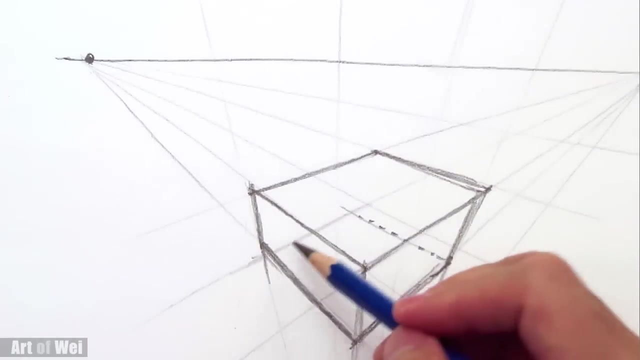 okay, and then let's just say: the bottom is going to be here, so make a relatively flat cube okay, so we connect that, all right, and then here for the back we can do so. this would be like this, this would be like this, and then this point here: 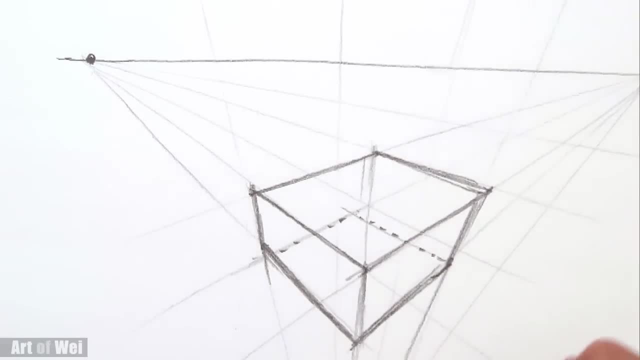 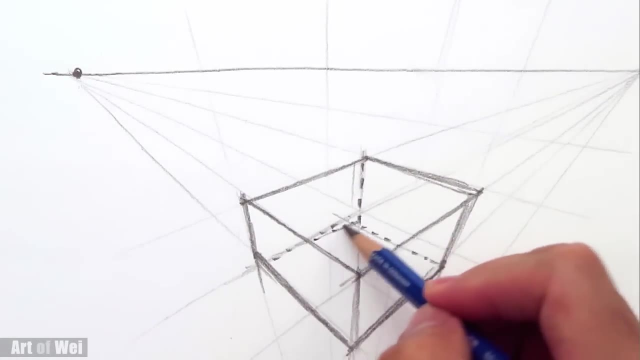 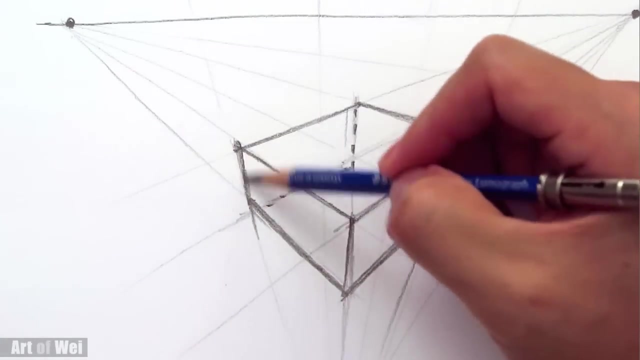 okay, here, actually this is a little bit off, sorry, so actually would be here. so if I had a ruler I can probably you know when you it'll be more accurate. but overall that's, it's close enough. so with three points perspective, you know, now you get this very. 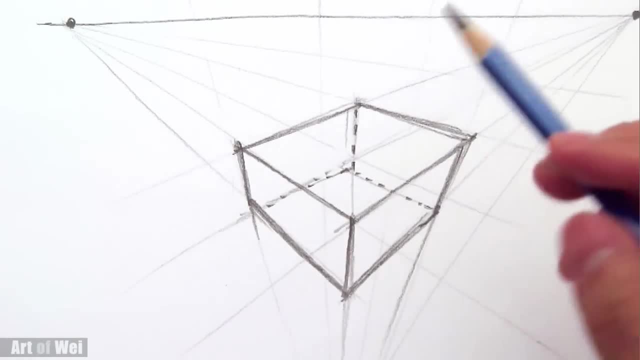 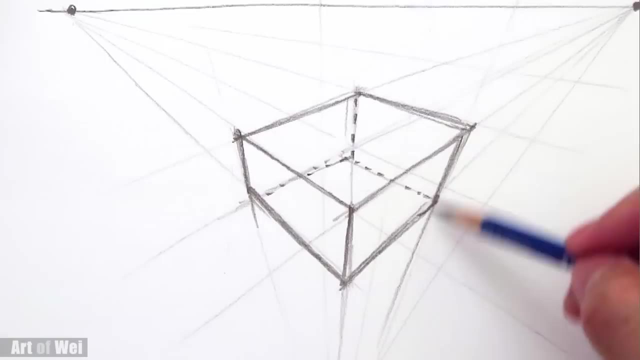 you know, dramatic perspective, but in general we don't use this a lot because with drawing it's just. this is a little bit too complicated and, seriously, if you want to do something like this, there are better ways to do it, but I'm going to show you how to do it in a little bit more detail. 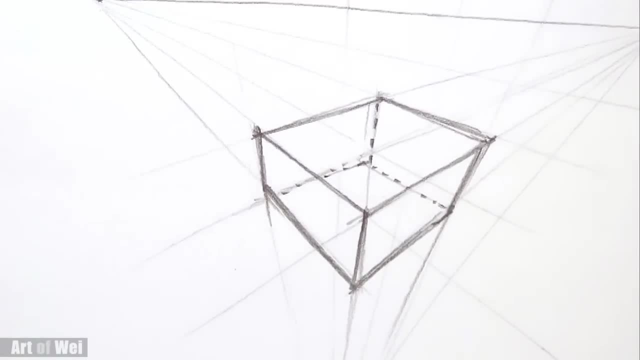 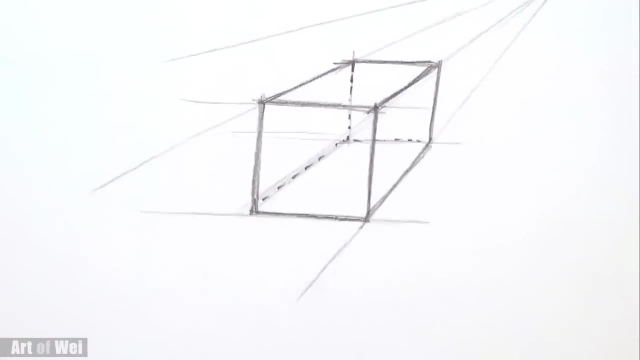 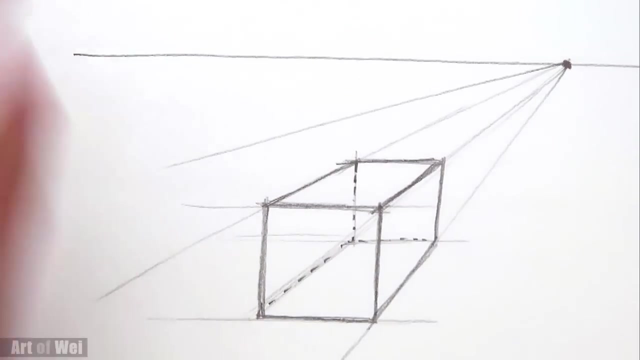 to lay out this kind of perspective and actually, you know, using 3d programs it's a lot easier. so, overall, so this will be your one point perspective- and this is very simple. when you're drawing, you probably want to make it a little bit more complicated than this- and two point perspective. 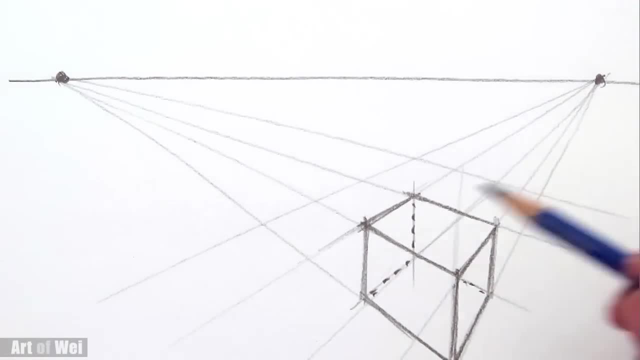 and this is, you know, probably the perspective that you want to use when you're drawing, because there's a. it's just a lot more dynamic. you know when, whenever, when there's kind of you know multiple angles, you know you can just kind of you know multiple angles and you can just kind of you know. 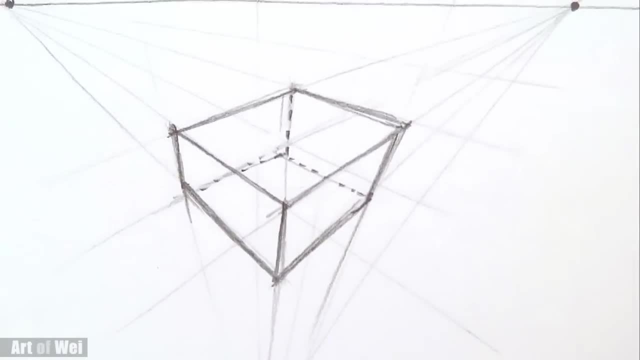 what's going on. and then three point perspective. yeah, you know, it's good to know, but generally we really don't use this much at all. all right, so to practice this kind of perspective. obviously, when we're drawing, you know we generally don't put these perspective line because it's just a little. 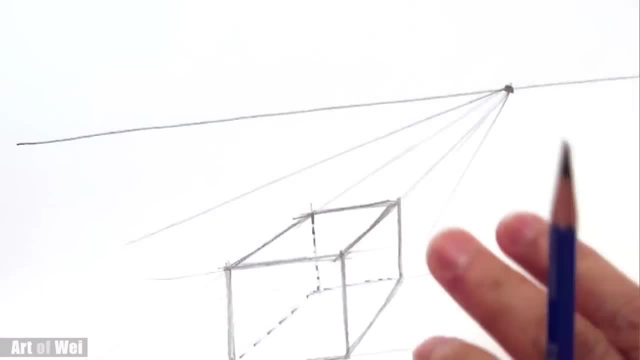 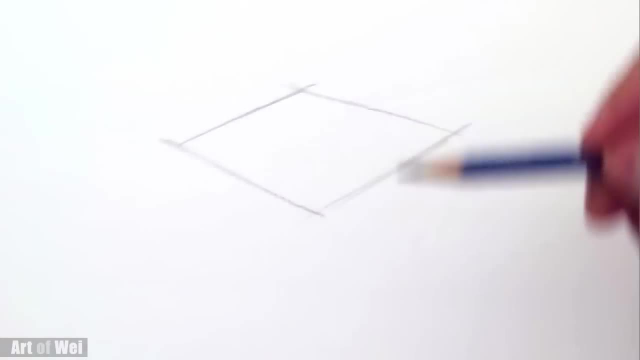 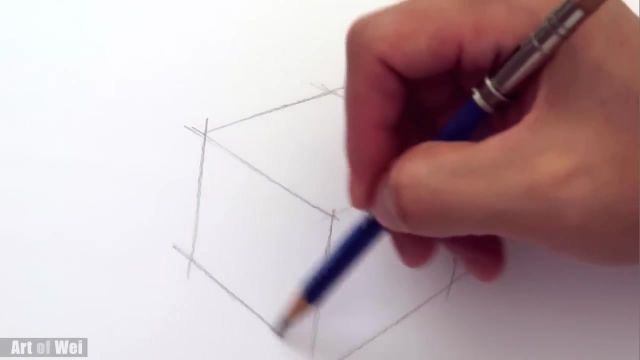 bit too much of a hassle, right? so let's say you want to draw a box freehand. you know it's very good to practice this kind of stuff. let's say I'm gonna- I'm just gonna- do a freehand, but do kind of a little bit of a two-point perspective and I'll show you why. you know you kind of have no, you kind. 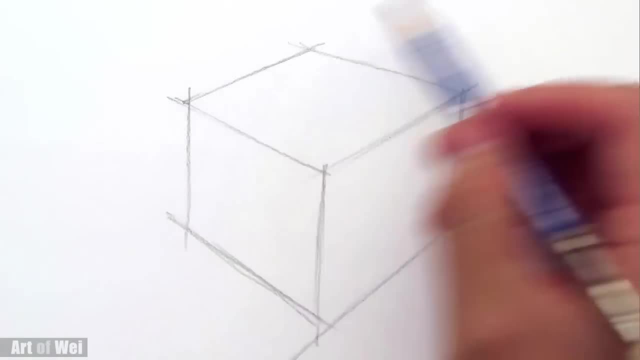 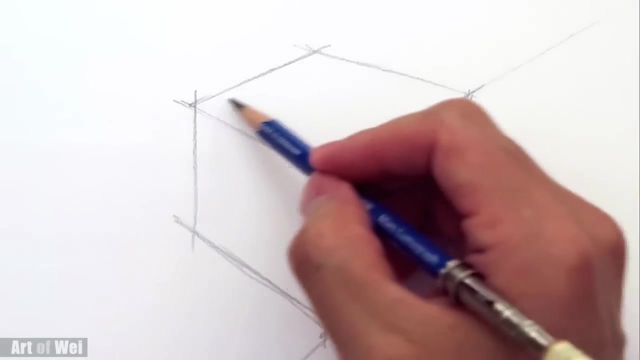 of want to do this kind of stuff freehand as opposed to working with vanishing points. so it basically, you know, with the vanishing points, you see, with this box, if I extend these, you know these will pretty much go off the paper. I mean, there's no, there's. you know the vanishing point is too. 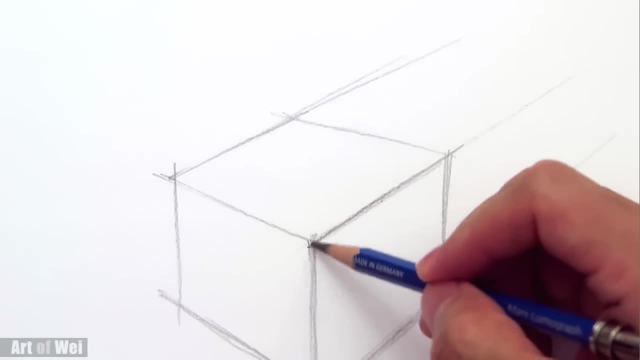 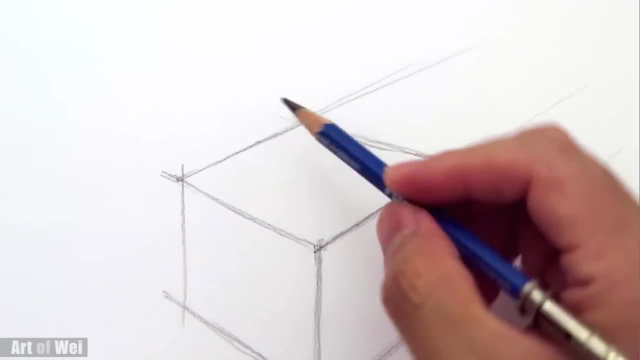 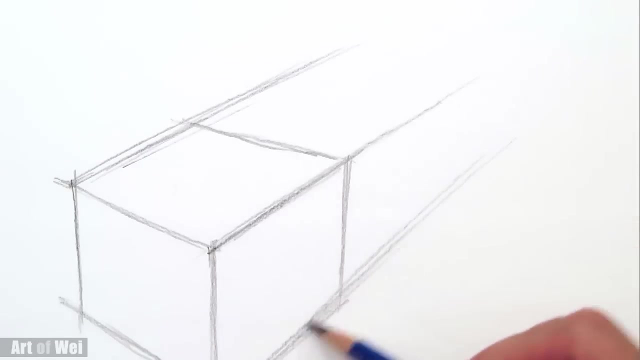 far away, right, because the perspective isn't- it's not that steep. so you kind of want to practice doing these kind of boxes and just kind of try to visualize that all these it's gonna go into a- you know that that vanishing point- and you want to be able to do. 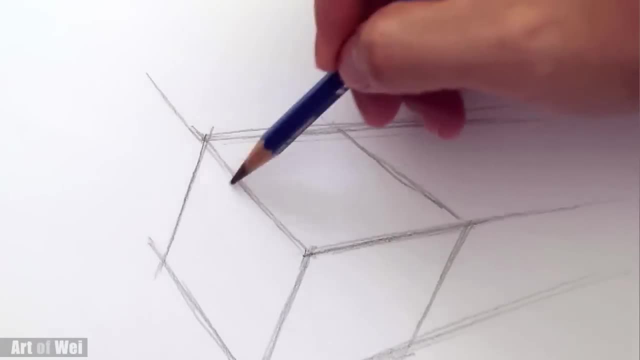 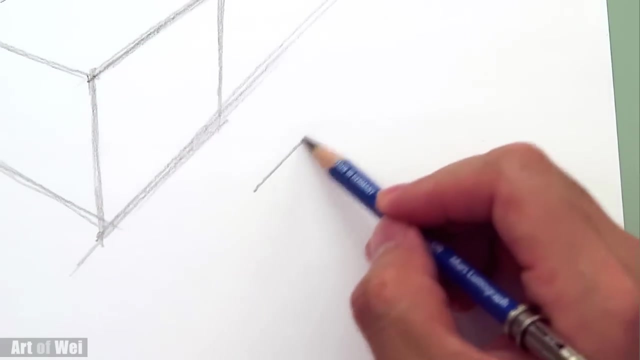 that kind of you know semi convincingly, so that you know kind of like, what I'm doing here. it's not super accurate, but it's kind of good enough. right, you feel like it is a box. I mean, if you're doing like a, like a box and you end up doing something like I don't know, you know you're gonna. 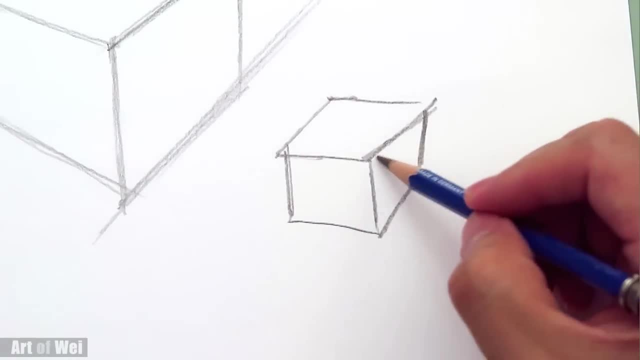 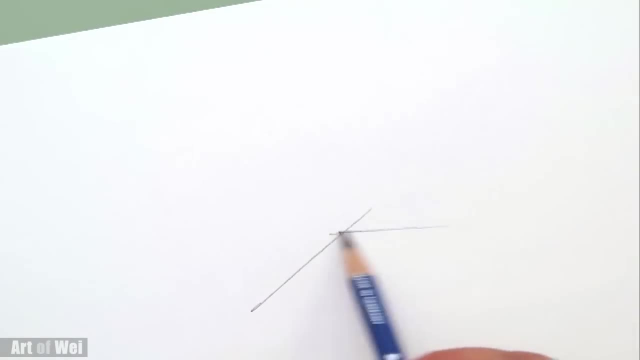 do something like that, you know, then something is weird, right, it looks like it's warped. so get into a habit of just kind of roughing in lines and you can even just do like a simple, just a little square on the floor, all right, and just try to visualize these lines going back like: 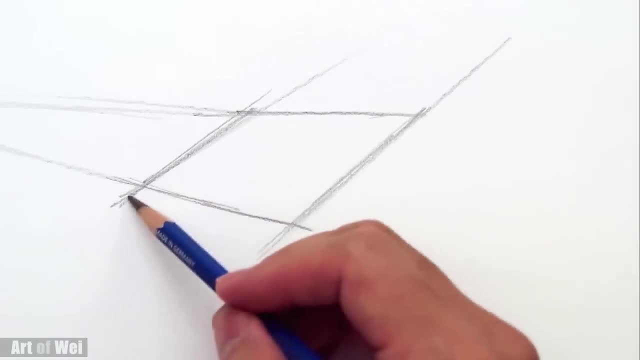 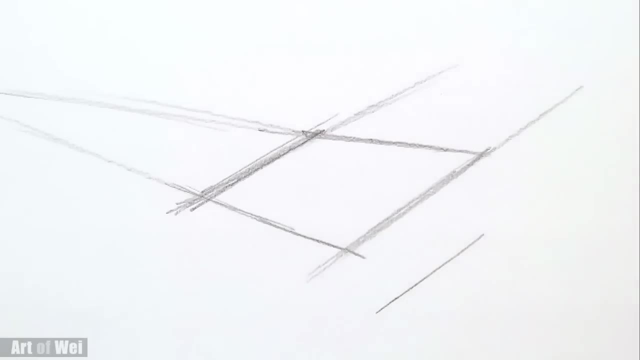 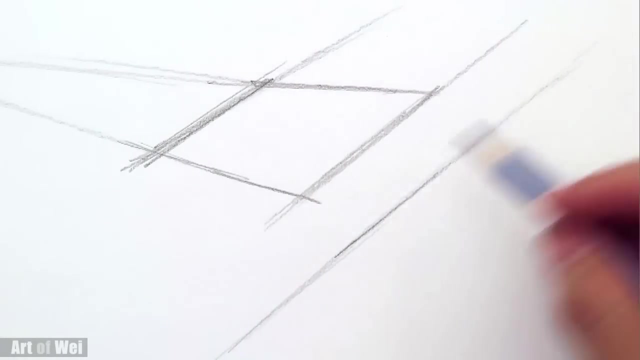 this one's a little bit steeper, and then this one. so that's why, when you're drawing, you know you, you generally don't want to draw a line and stop. you know, with linear lines it's just kind of just go over it. you know, let it, let it go past you, you know past what you want to draw, and that's. 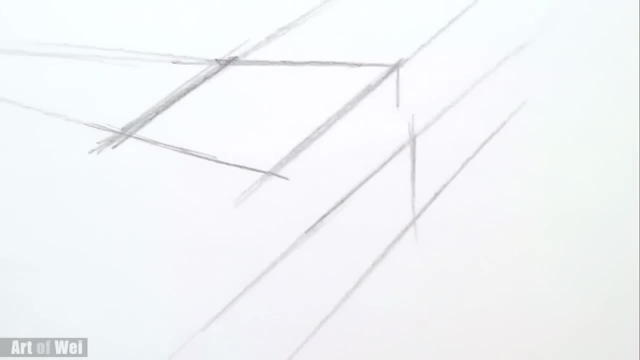 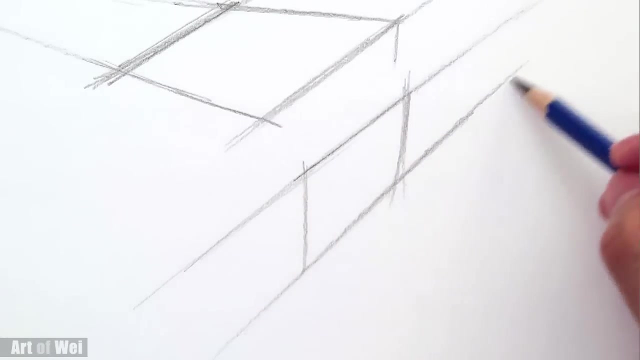 really helpful in trying to visualize that way. you can visualize the perspective right, because once you extend the lines and you gotta be able to see, oh, you know that this is not correct right, or the angle is wrong. so like, if I do something like this and now we know, you know this, this line doesn't.